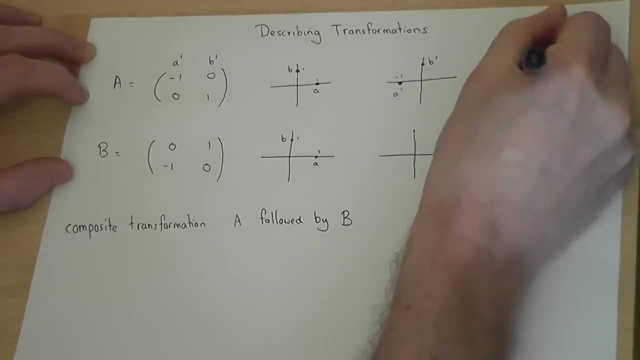 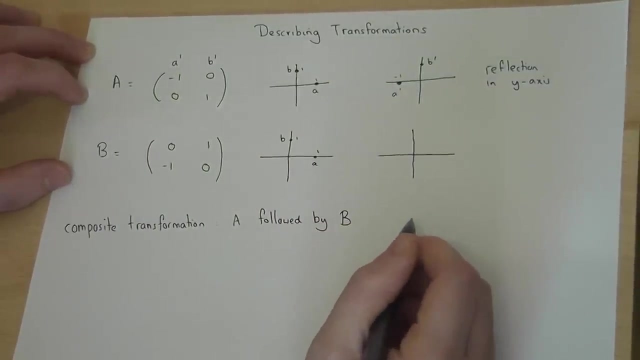 So a represents a reflection in the y-axis. So to elaborate this further with a second example, consider b Again. the first column is what happens to a? That's a dash. The second column is what happens to b? That's b dash. 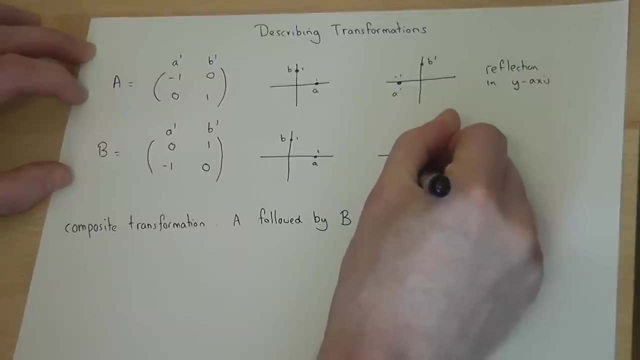 So a has gone to, which is down here, And b has gone to, which is across here. So what you can see is this L shape has basically rotated round by 90 degrees. So we have a rotation of 90 degrees and it's clockwise. 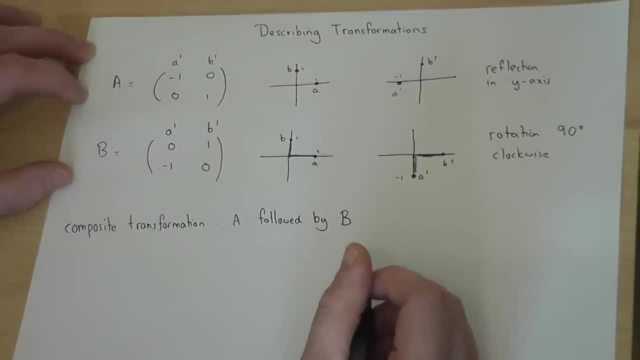 So they're two separate transformations And those golden rules about what happens to a and b always applies to any matrix. We can also have composite transformations- a followed by b- And we can work out the single matrix to represent this by doing the following: 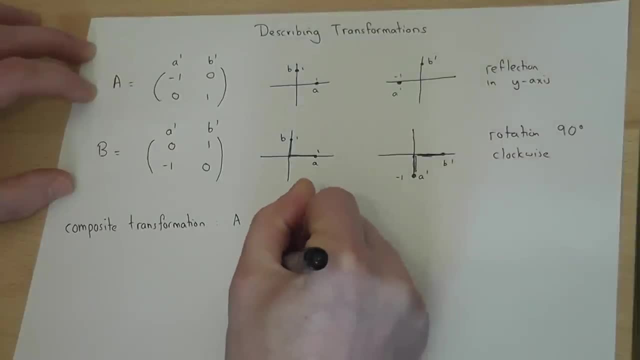 We begin with a and we follow it with b and we follow from the left, So a followed by b. That's quite key that we keep that order. So we've got to work out what b times a is. So if we times together those two matrices, 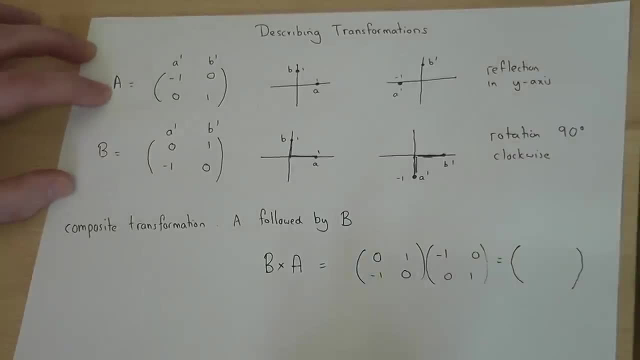 we get the single transformation which represents that: So 0 times minus 1 and 1 times 0 is 0.. 0 times 0, 1 times 1 is 1.. Minus 1 times minus 1, 0 times 0 is 1.. 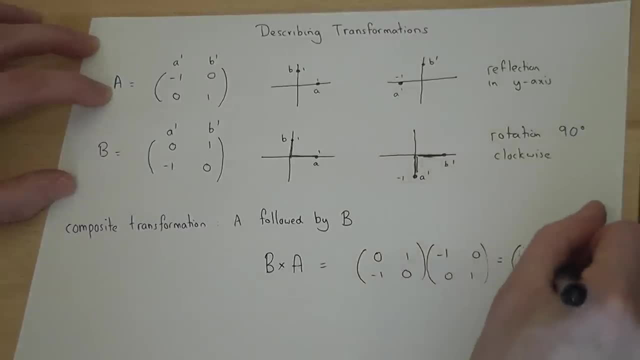 And minus 1 times 0, 0 times 1 is 0. And the question could be is: what does that represent? Well, this is a dash, This is b dash. If I draw a quick sketch, a dash has gone to 0, 1..